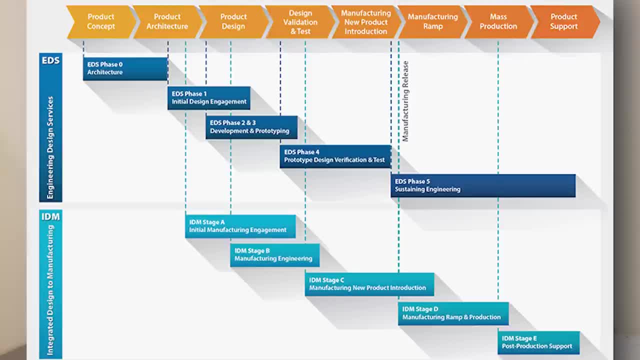 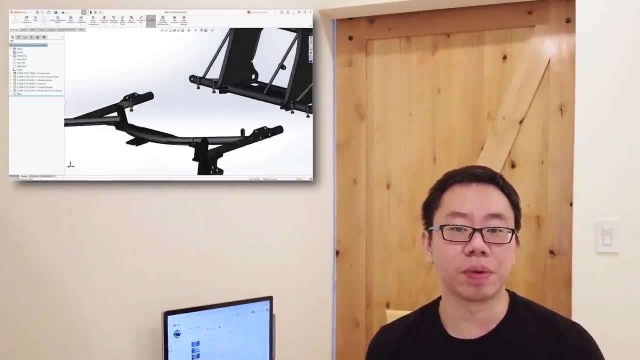 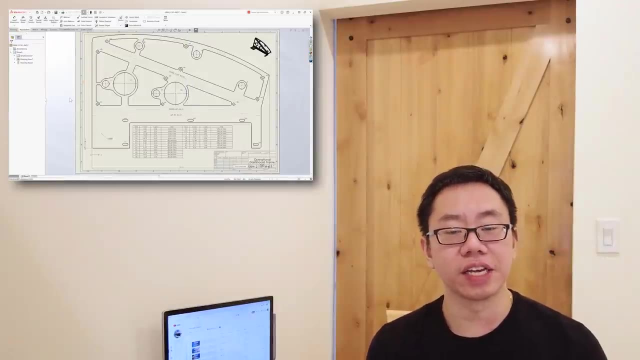 high-volume manufacturing phase of the product development process. Throughout this entire process, you'll use CAD software to design and create hundreds, if not thousands, of parts, sub-assemblies and a top-level assembly, and eventually two-dimensional drawings of all of those parts so that they can be produced and assembled. There will without question be 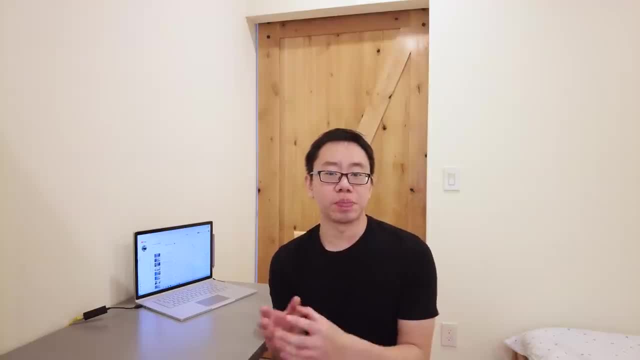 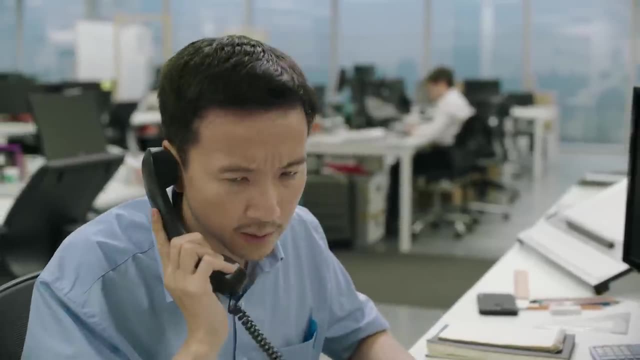 multiple revisions of each part of the product If you're interested in learning more about CAD. as you begin to test prototypes and discover the weaknesses in your design- and it's very likely that your boss, industrial designers and the marketing team will tell you that your design 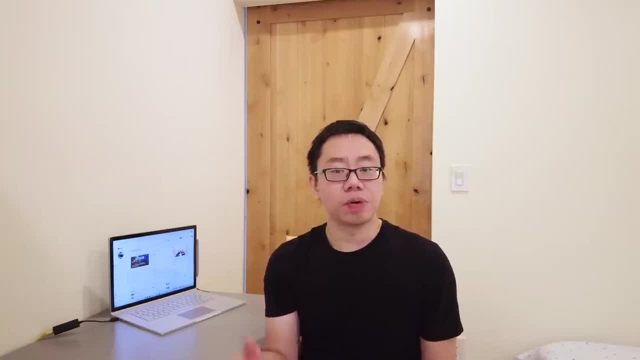 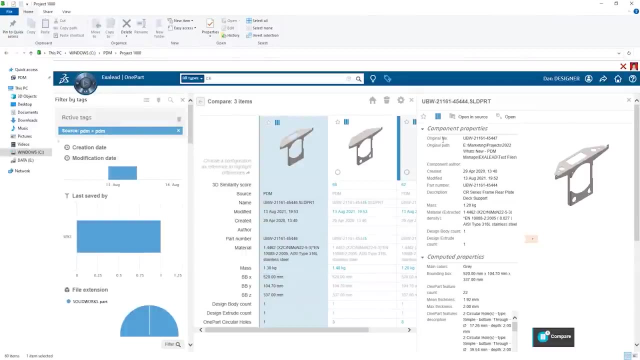 is garbage. As a mechanical engineer, part of your job will be to keep track of these revisions using CAD and revision control software, and to communicate these changes to your internal team, as well as your vendors and manufacturers, so that everyone is on the same page. 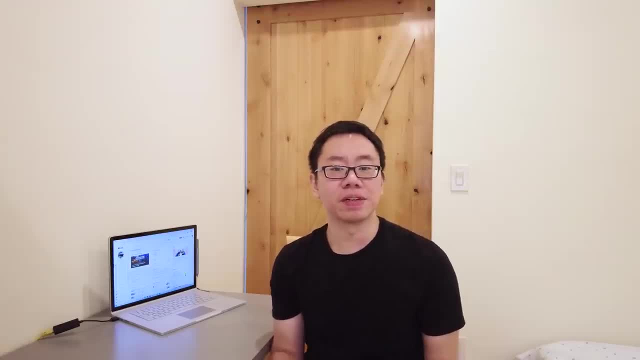 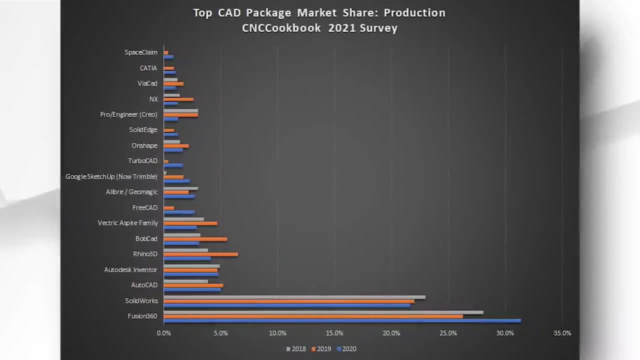 Now, over the past 20 years, many companies have developed CAD software, some of which are exceptional and others not so much So. the most popular ones, according to this survey conducted last year, include Solidworks, Fusion 360, AutoCAD, Autodesk, Inventor and Rhino. 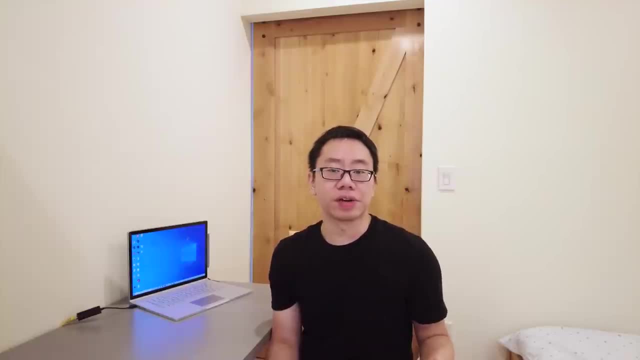 3D. However, keep in mind that a lot of industrial designers, as well as other types of engineers, like electrical, civil and industrial, also use CAD, so I'm going to eliminate most of these and only include the ones that mechanical engineers use. based on company, The Solid Systems makes two. 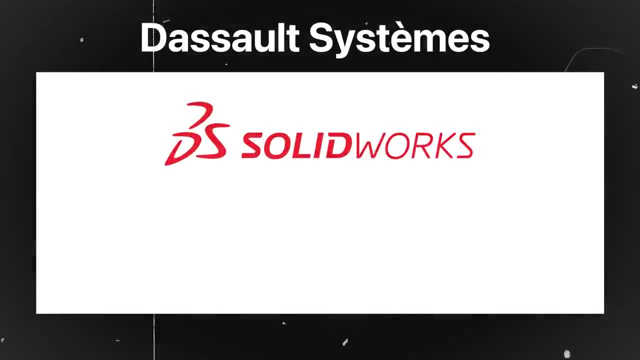 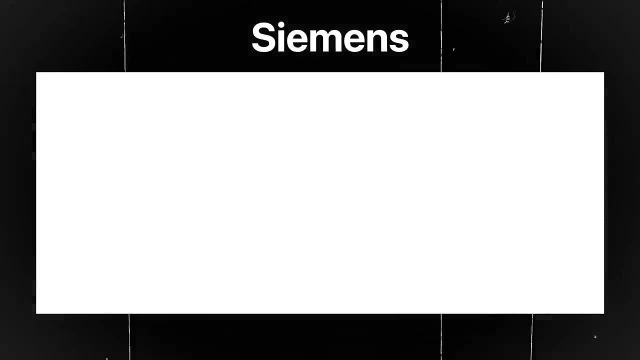 most reputable CAD software, including Solidworks, and the less popular one, Katia, which I like to think of as a higher-end version of Solidworks. Like the Solid Systems, Siemens also makes two CAD software: Solid Edge, which is rarely used anymore, and a higher-end version called NX. 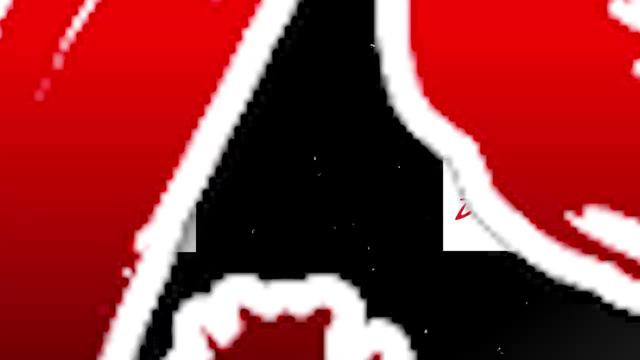 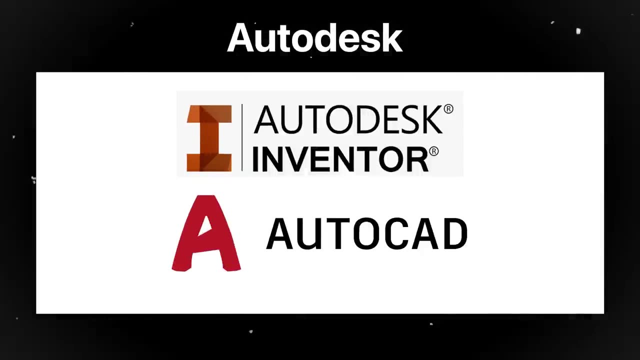 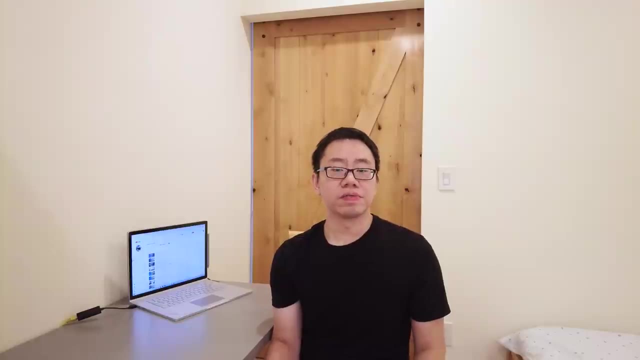 PTC makes Creo, which is also very popular and competes directly with Solidworks. The last two are made by Autodesk and are a lot less popular but nonetheless still used by mechanical engineers, and they are Inventor and AutoCAD. All of these softwares have similarities and differences, but they all serve the same exact. 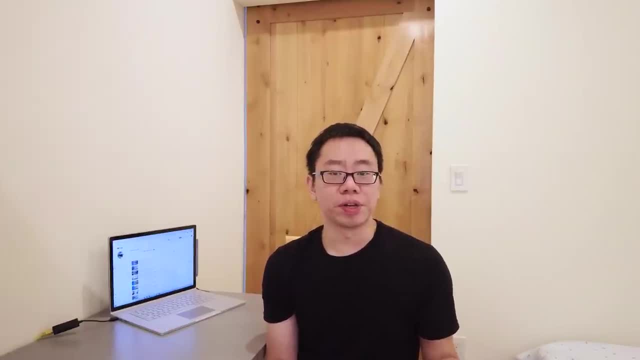 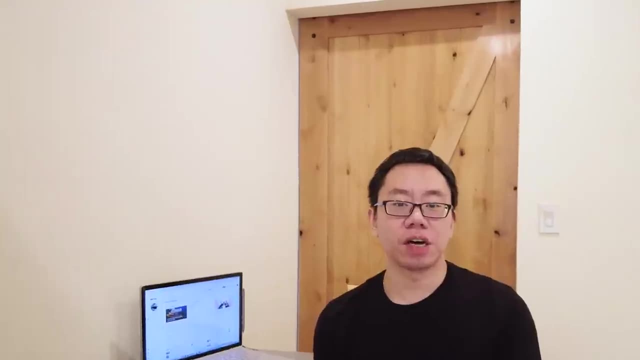 function and which one you use really depends on which company you work at, which could very well be two or more of these softwares. Now I made a video a while back looking at which CAD softwares the Fortune 500 companies use the most and if you're interested in seeing the results, 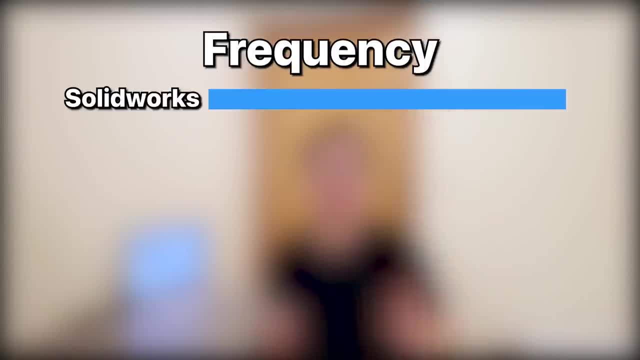 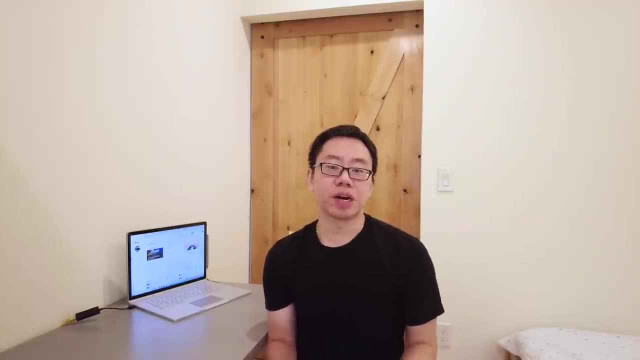 go ahead and click here. Solidworks appeared the most times in these companies' job postings, followed closely by Creo. We also saw that Katia and NX are commonly used in the aerospace industry, at places like Boeing, Lockheed Martin and General Dynamics. 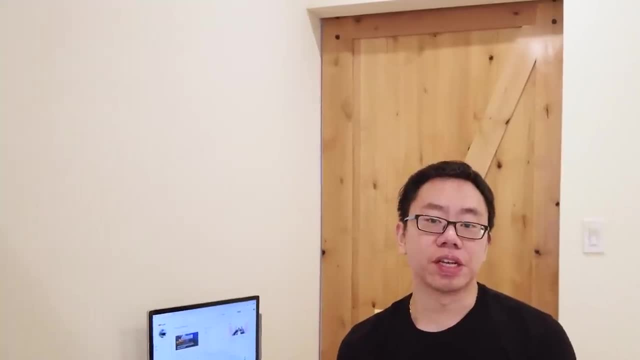 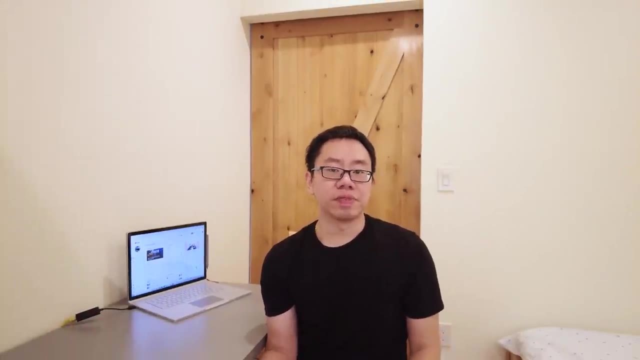 NX is also commonly used in the automotive industry, at places like Ford and GM, as well as rich companies like Apple. On the opposite of the spectrum, AutoCAD and Autodesk Inventor appeared in none of these job postings, So what I would recommend to you guys is learn either Solidworks. 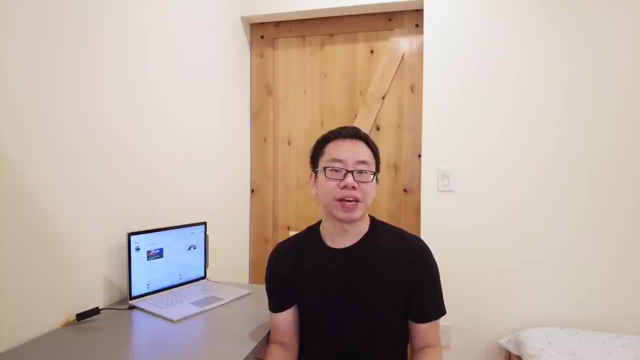 or Creo. Both are great and you'll have no issues picking up Katia or NX if that's what your future employer uses. Last thing I want to mention is developing a mindset for designing parts that are robust, ergonomic, manufacturable, cost-effective and can be assembled easily matters way more to. 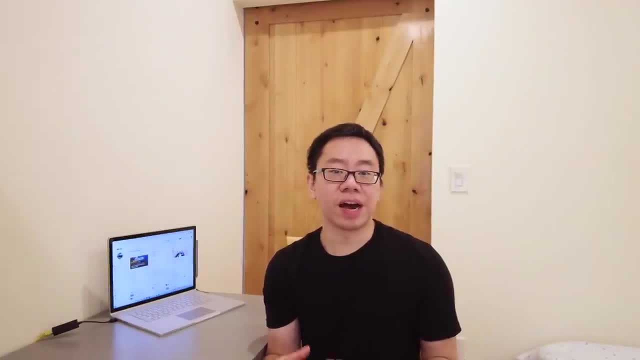 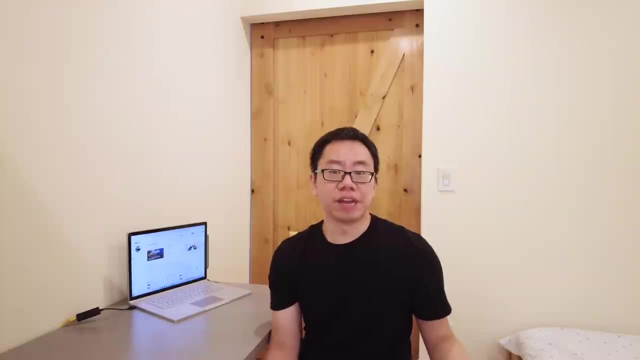 employers than which software you actually learn, And good hiring managers know this, so they won't filter you out just because you're, say, good at Solidworks and unfamiliar with Katia, And if they do, you probably don't want to work for them in the first place. Next is numerical simulation, or CAE. 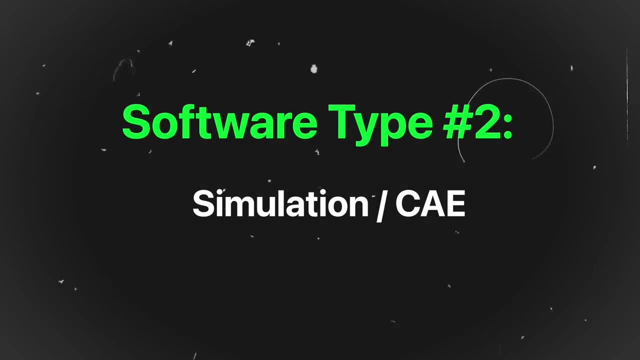 computer-aided engineering software. Next is numerical simulation or CAE, computer-aided engineering software. Next is numerical simulation, or CAE, computer-aided engineering software, Which you will 90% be using at some point in your career As a mechanical engineer. you will have opportunities. 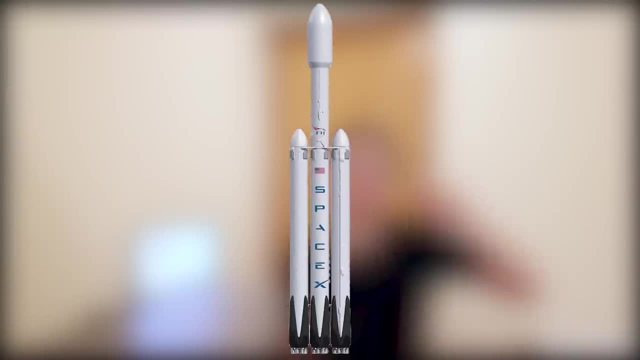 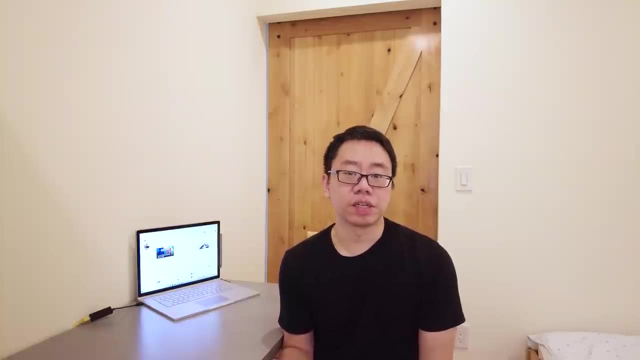 to design something as small as an Apple Watch to something as big as a SpaceX Falcon 3 rocket. using Kat's software, You'll also have to come up with tests to validate the strength, durability, performance, functionality and safety of your design concepts throughout the entire product. 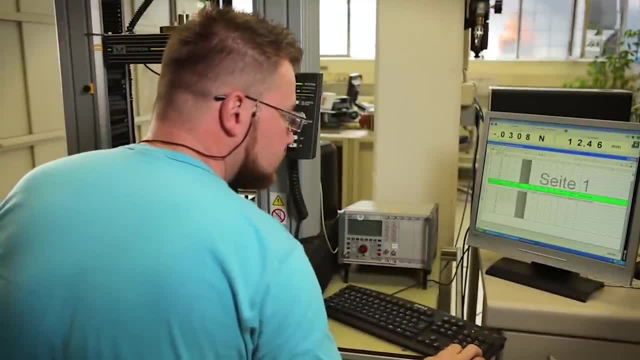 development process. For example, tests you would generally perform in the late stages of the product development process for consumer electronics. For example, tests you would generally perform in the late stages of the product development process for consumer electronics. For example, tests you would generally perform in the late stages of the product development process for consumer electronics. 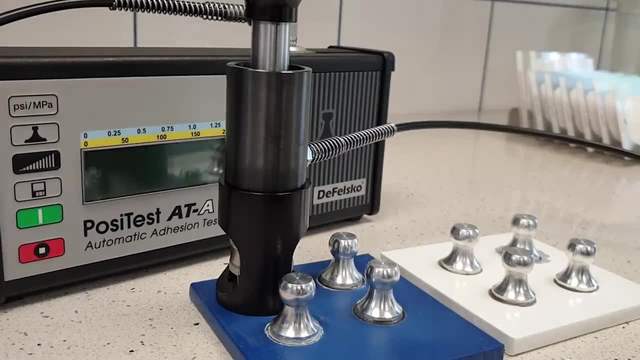 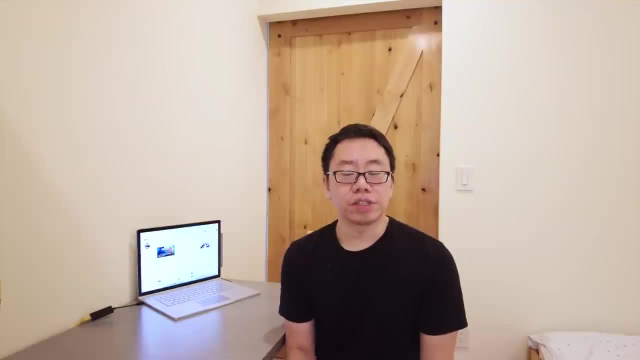 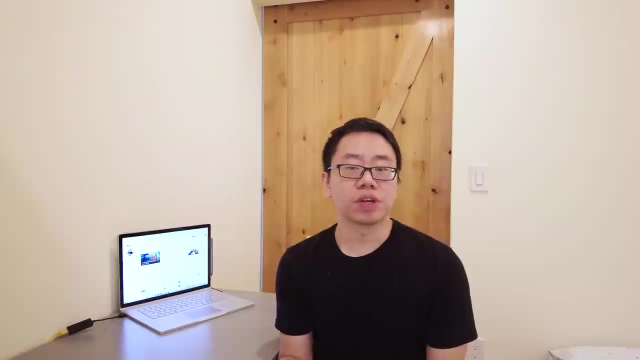 Include dropping the product from various heights, push and pull testing, vibration testing, battery testing and ingress testing. However, mechanical engineers need to predict the behavior of their designs and prototypes way before the testing of the final product. So this is where CAE software comes in and plays a critical role in saving both time and 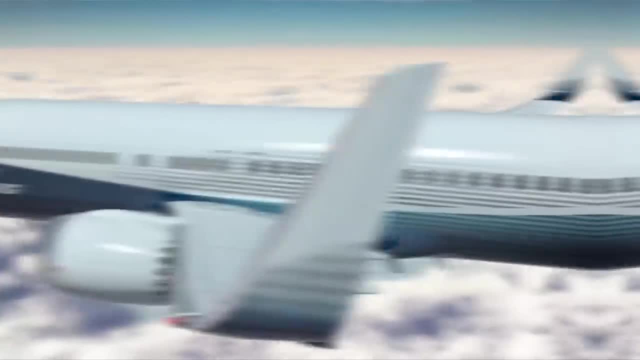 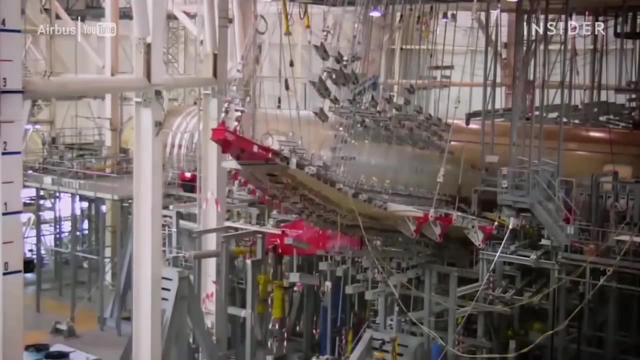 money for an organization. You might be wondering what I mean. Well, say, you are designing the parts in an aircraft wing Instead of building and testing thousands of prototype designs in a lab to find out which configuration yields the lowest stresses, which in itself might take you well over. 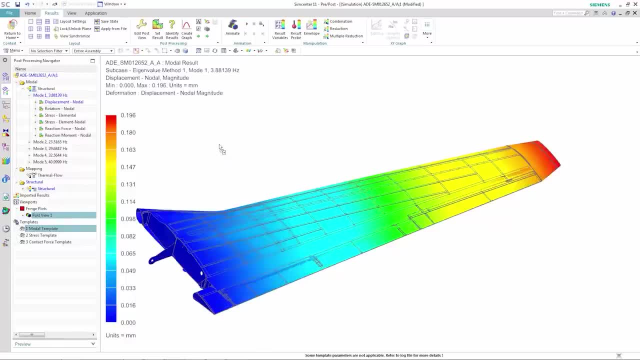 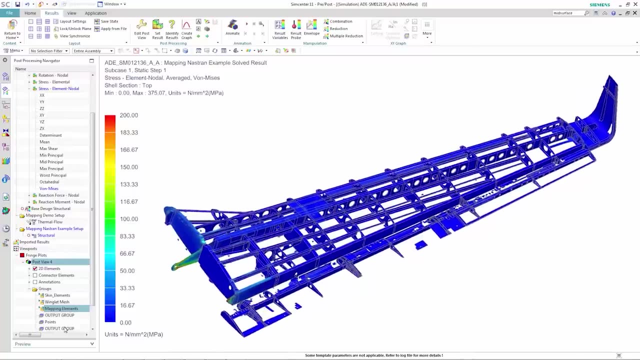 a year and cost a fortune. you would set up simulation models using finite element or FEA software to conduct a design of experiments and iterate through various design parameters and ideally arrive at an optimal solution within several weeks. At the same time, you could use 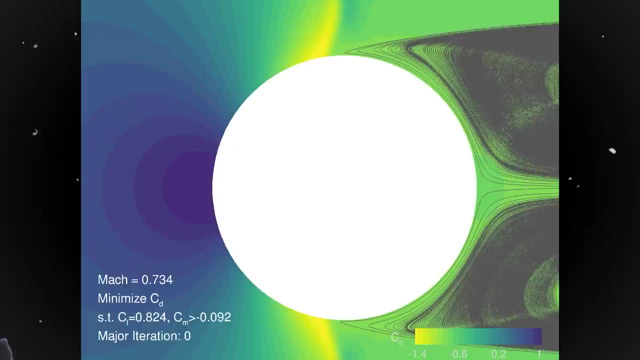 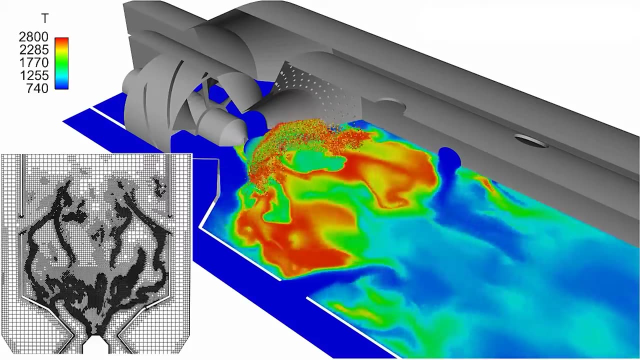 computational fluid dynamics, or CFD software, to optimize the way you design the aircraft wing. As you can see, CAE software is not meant to replace real-world testing entirely, but rather seeks to complement it and shorten the product development process. So there are two categories. 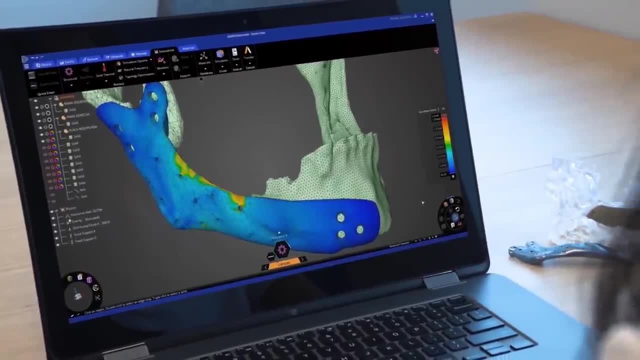 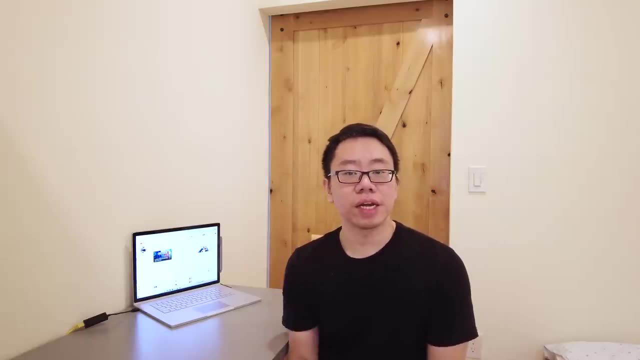 of simulation software. The first category is embedded into your typical CAD software, such as SOLIDWORKS and CREO, And the second category is standalone simulation software which is designed to optimize the thermal management system of the jet engines. So the first category is 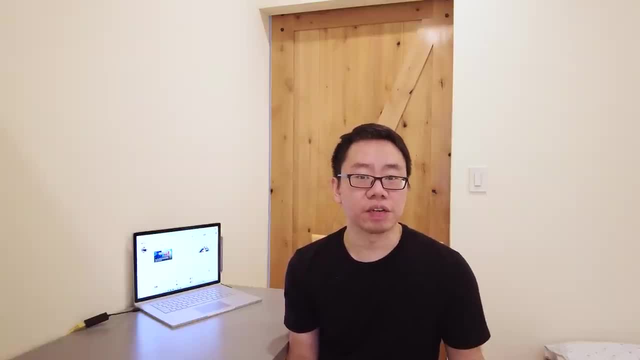 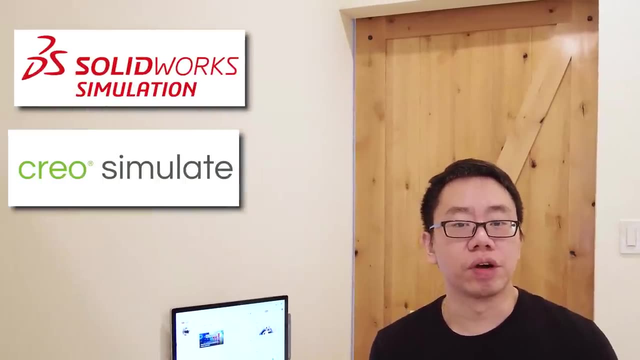 embedded into your typical CAD software, such as SOLIDWORKS and CREO. And the second category is standalone simulation software which is designed to optimize the thermal management system of the jet engines. So the first category is embedded into your typical CAD software, such as SOLIDWORKS and. 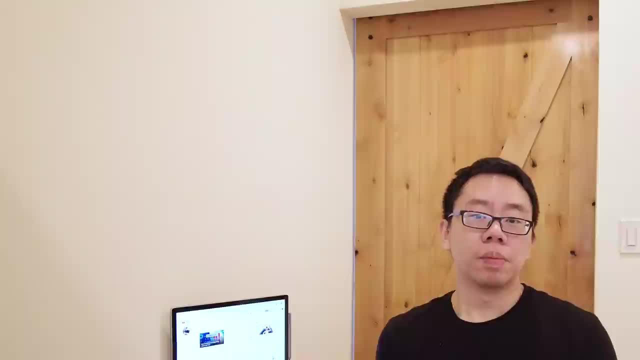 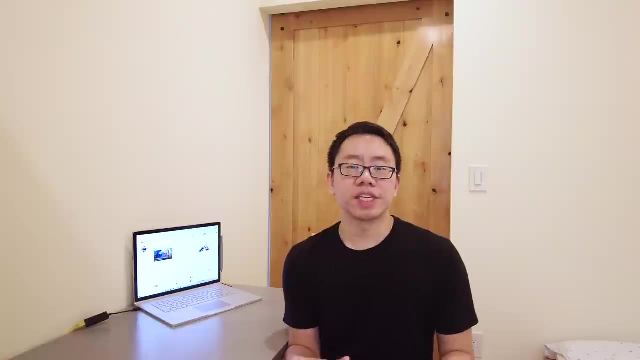 CREO. And the second category is embedded into your typical CAD software such as SOLIDWORKS and CREO. Both software are user-friendly enough to get a good feel for what it's like to set up a FBA or CFD problem, which can seem overwhelming at first because of how involved it is. 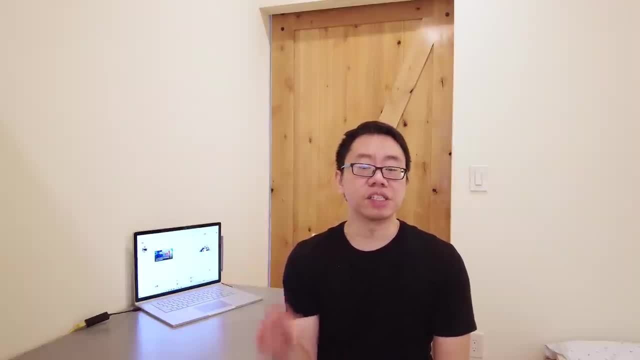 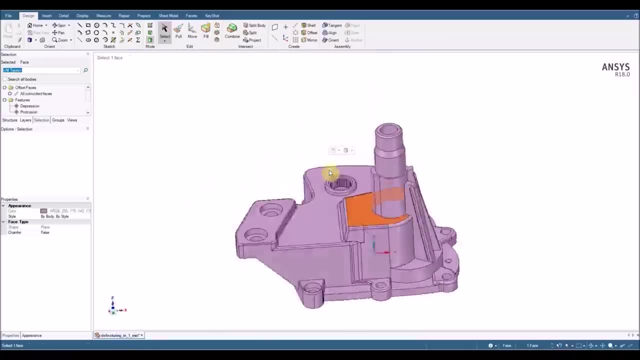 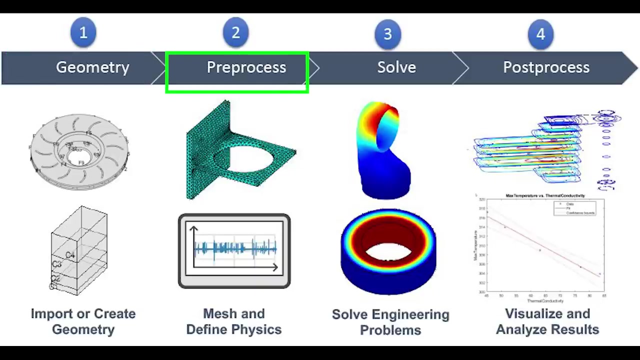 Setting up any CFD or FBA simulation consists of four key steps that i'll briefly walk through. the first step is geometry, which involves cleaning up features in the cad model that are difficult to mesh and importing your cad model. the second step is pre-processing, which involves meshing and defining all of the physics, such as boundary. 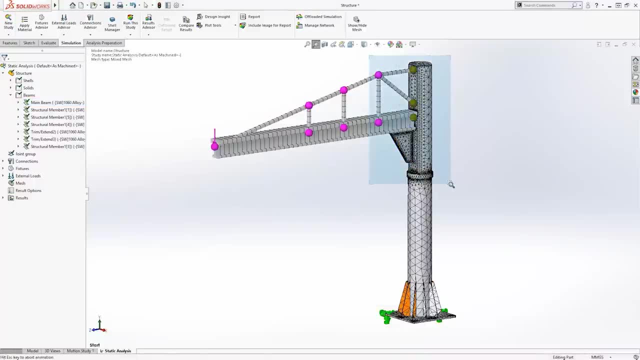 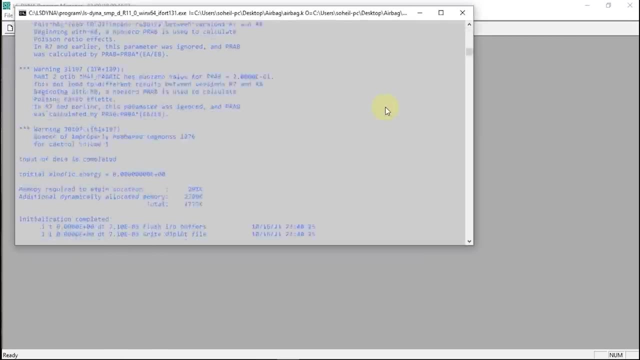 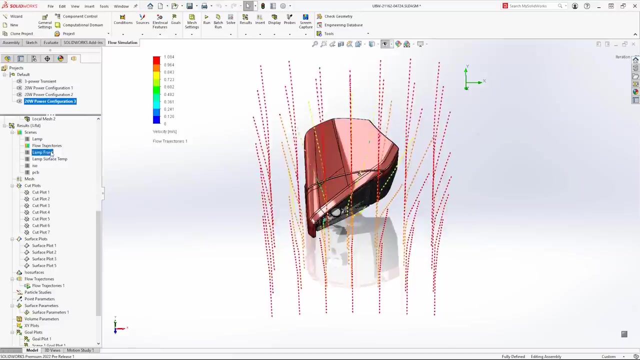 conditions, forces, and selecting the right material or turbulent models, depending on whether you are simulating solids or fluids. the third step is solving, where you initiate the simulation for the computer to solve, and the fourth step is post processing, where you visualize and analyze the results to see if they actually make any physical sense, as i mentioned before, which cad software you 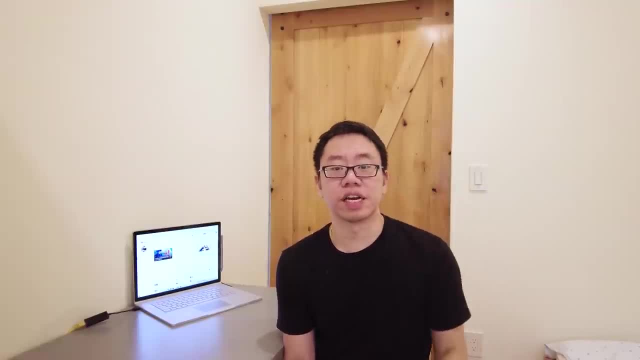 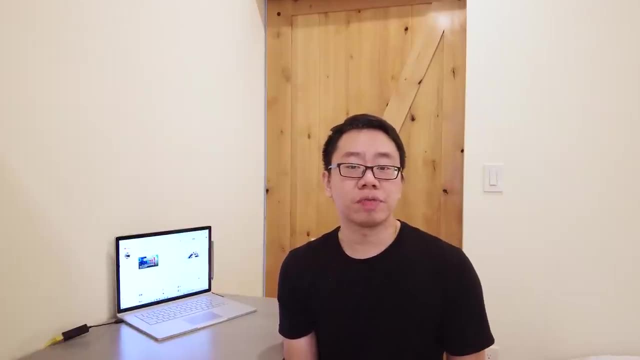 learn is not as important as developing an intuition for designing parts that are manufacturable, cost effective and ergonomic. the same goes for cae software. which software you ultimately learn doesn't matter as much as knowing how to accurately set up an fpa or cfe simulation. make the right 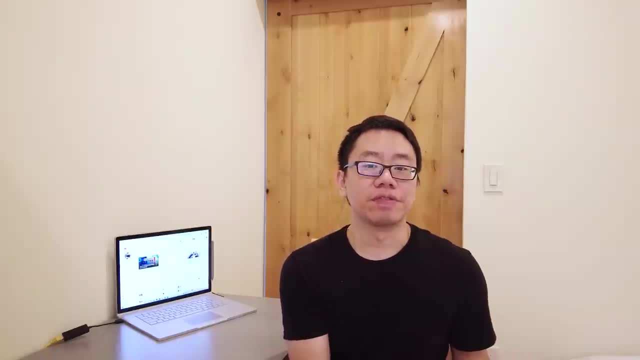 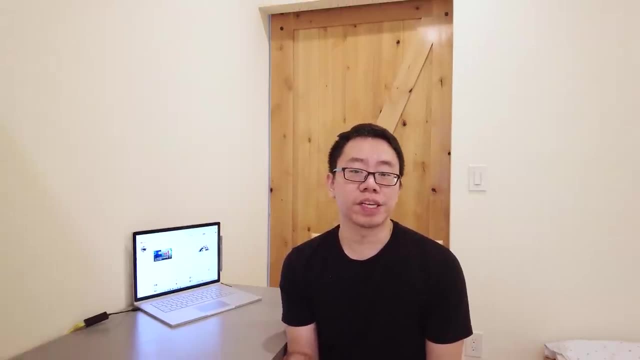 assortment of software that you can use to make the right assortment of software so that you can assumptions and gauge if the results are in line with the physical world, following the four steps that I mentioned. Only when you have mastered and feel comfortable setting up problems in SOLIDWORKS. 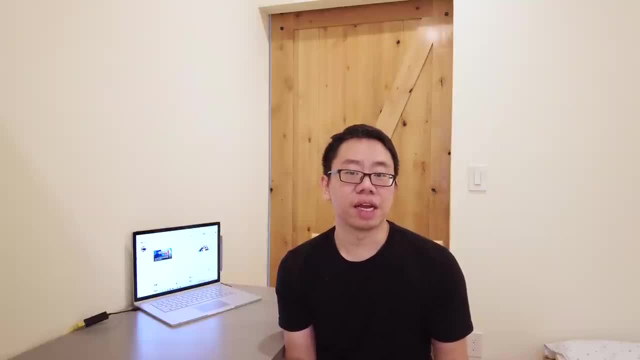 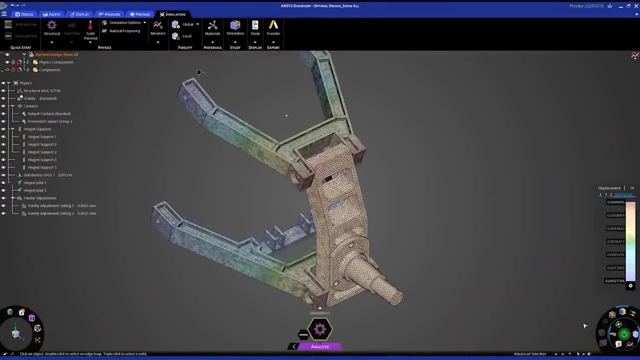 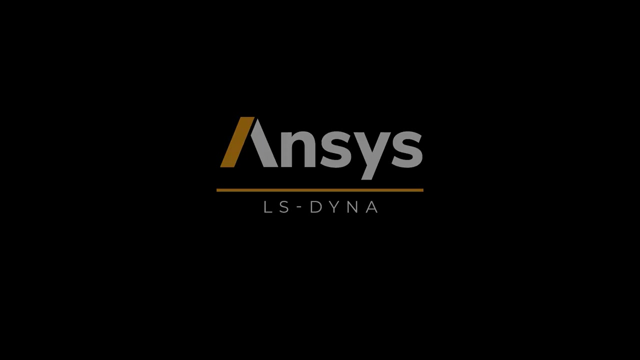 or Creo Simulation, would I recommend you to try out the standalone CAE softwares such as ANSYS. ANSYS is one of the most popular and powerful standalone FEA and CFD softwares used in industry to simulate both linear and non-linear problems. ANSYS also recently acquired LS Dyna, which is a 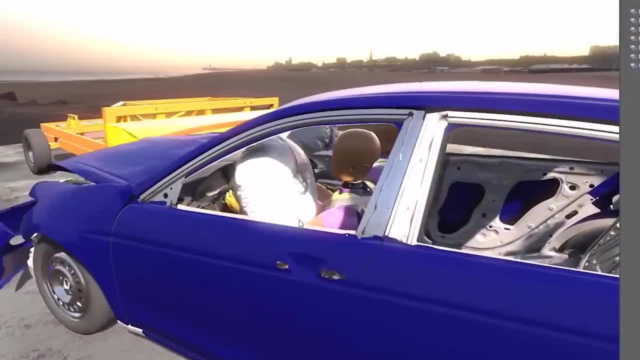 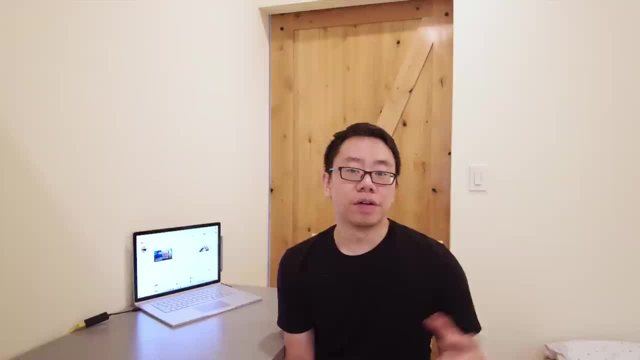 high-end FEA software that I used myself in grad school to simulate automotive crash and impact problems and is a valuable asset to have if you're planning on working in the automotive industry. Finally, another very versatile and powerful software, very similar to ANSYS, that I strongly 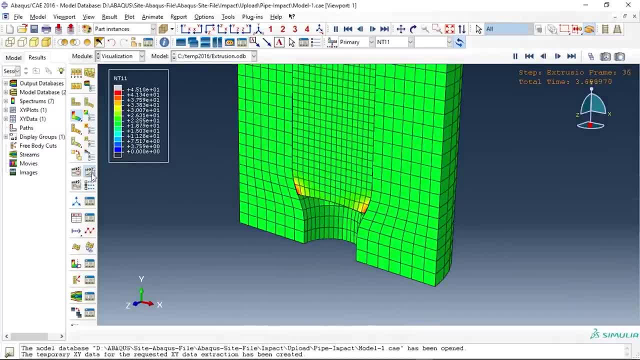 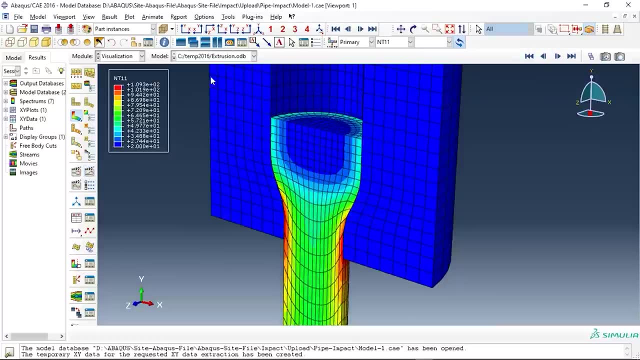 recommend is Abacus. Abacus is used at many of the fortune 500 companies like Amazon and is great for simulating linear and non-linear static thermal dynamic and impact effects, as well as fracture and failure behavior. Abacus is also used to simulate linear and non-linear static thermal dynamic and impact effects, as well as. 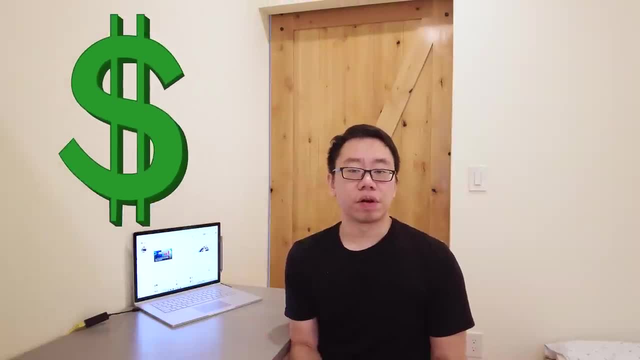 fracture and failure behavior. Keep in mind that these standalone CAE softwares are very pricey and run for about $30,000 or more per license, so it might be a challenge to get your hands on a full version, but I did do some research and all of them, surprisingly, offer a free learning edition for. 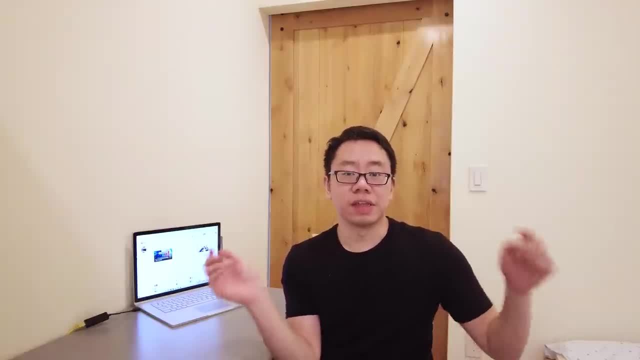 students, so if you're interested, definitely check out the links down below. The last thing we're going to talk about is programming and computational software. Being a mechanical engineer in the 21st century, where everything is going to be easy and simple, is technology-driven, AI-driven and automated programming, is, for sure, a nice skill to have. 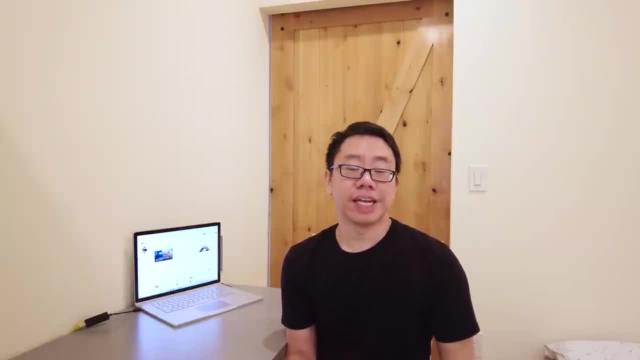 to complement your CAD and CAE skill sets. It's not a must-have skill, but it can without question make you stand out in a job interview or at work. if you can leverage your programming skills to automate a test process, a data analysis process or any process. really Knowing how to program will. 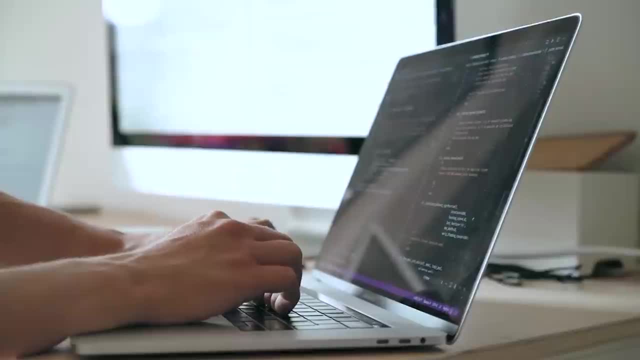 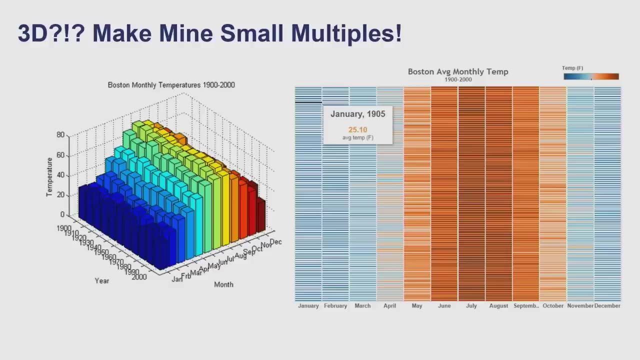 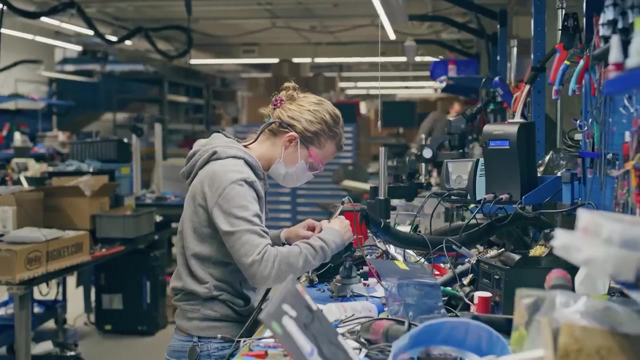 also increase your individual efficiency at work. In a matter of minutes you can perform very complex calculations, visualize and analyze test data and create beautiful plots for your next big presentation with senior executives. Programming is especially important for those of you who want to go into mechatronics, controls or robotics to program actuators and motors. So the programming. 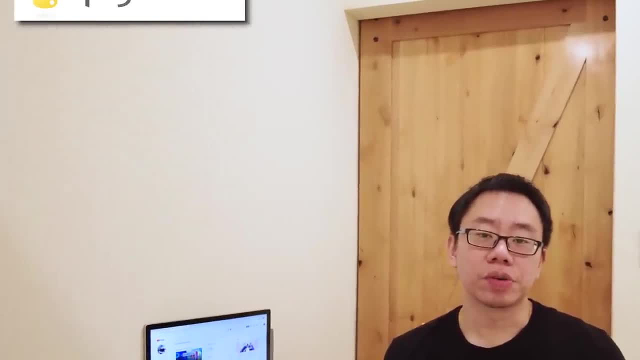 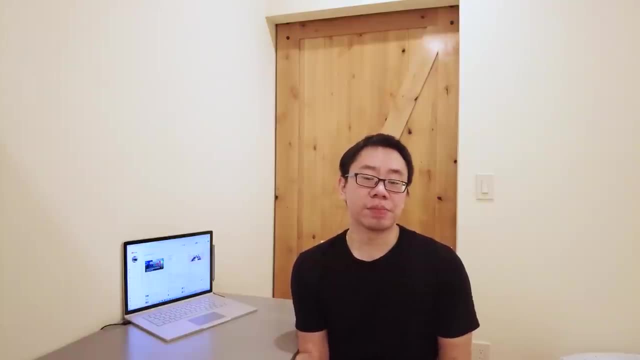 language I would recommend learning is Python. It's open source, very efficient, easy to learn and can be used for a lot of things. If you're a beginner, you might want to learn a little bit with just about any kind of application, from data analysis and machine learning to automation. 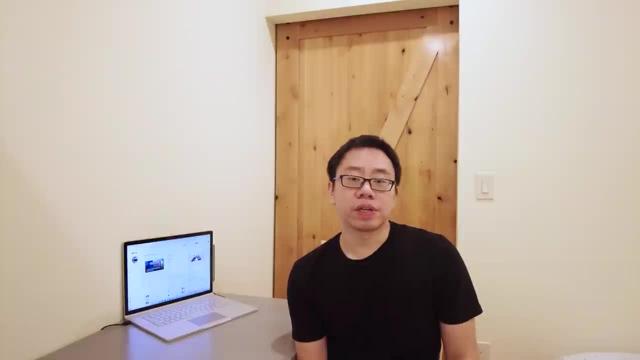 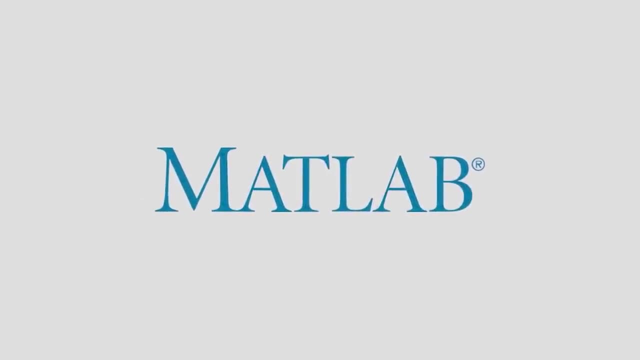 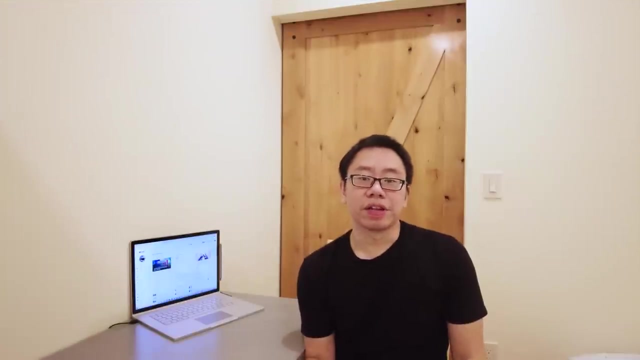 and motor control with the Raspberry Pi. I would only recommend learning C++ if you're serious about robotics, where performance matters. An alternative to Python is MATLAB, which is another very user-friendly programming language that I recommend learning if your school has licenses. However, it's not free like Python, so if your future employer doesn't use it, 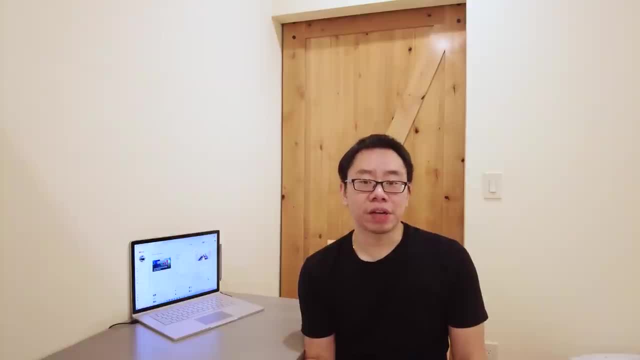 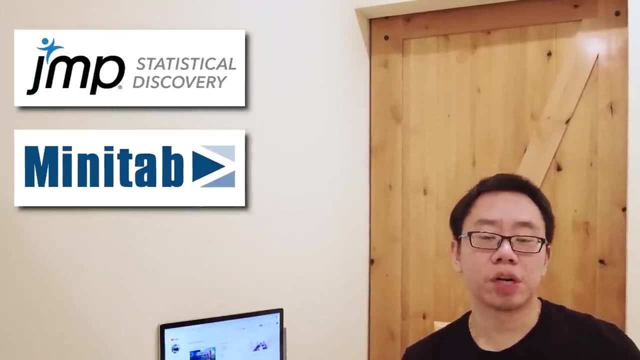 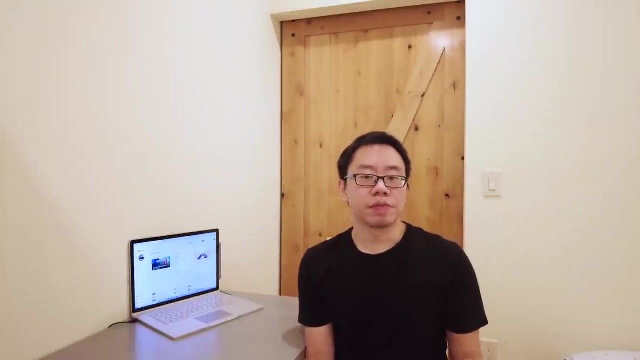 you'll be out of luck. So choose one to learn, preferably Python, but MATLAB is just as capable. Some other software that I had to use at previous jobs include Jump and Minitab, which are both statistical analysis software that offer a very intuitive user interface. Typically, you'll see many process manufacturing and 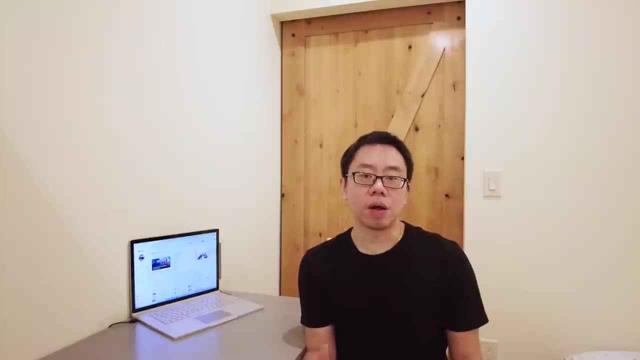 quality engineers use them for applications like Six Sigma, quality control, design of experiments and regression analysis. Now, I know Excel is always talked about and that mechanical engineers use it for quick calculations and making plots, but please don't write it on your resume. It only acts as a filler and makes you look bad If you're an engineer. 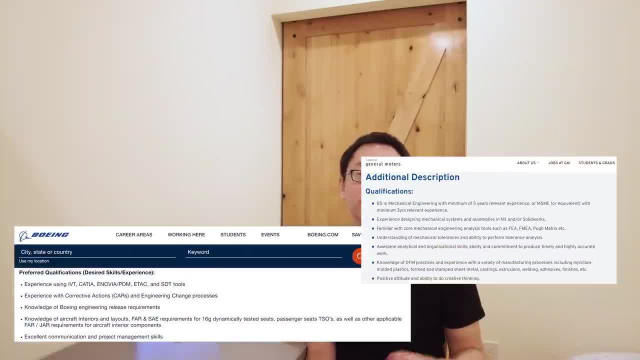 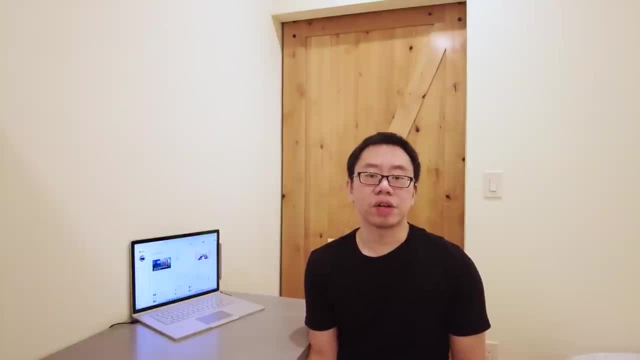 it's a given that you know Excel, and that's why you never see it listed as a requirement in any engineering job posting. Finally, there are a couple graphical programming languages that are good to learn if you want to become a control systems or test engineer. 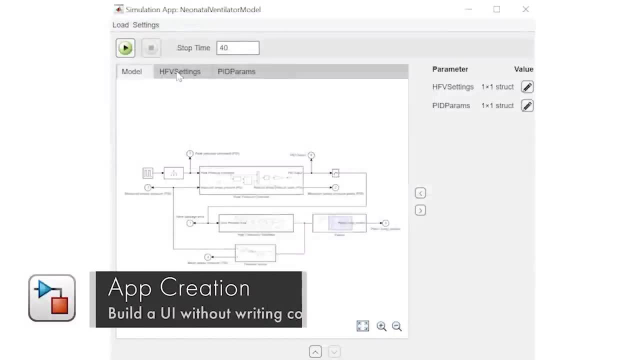 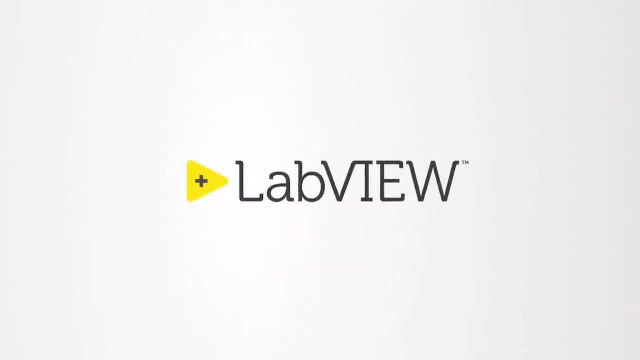 First is Semilink, which is integrated into MATLAB and is used to model, simulate and analyze dynamical systems like the cruise control system of a car. Second is LabVIEW for high-speed data acquisition and control in a test lab or specialized manufacturing. 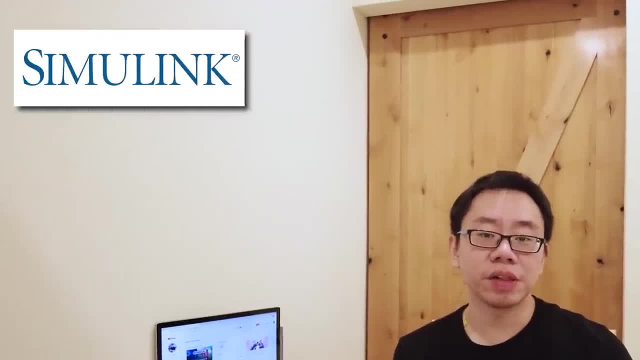 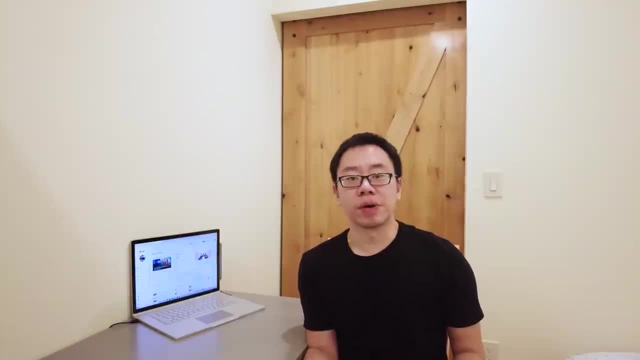 processes. So if you're interested in control systems, then Semilink is a great way to go, And if you want to do more product testing involving data acquisition systems and controlling equipment and instruments, then LabVIEW is without question, the best software to learn. 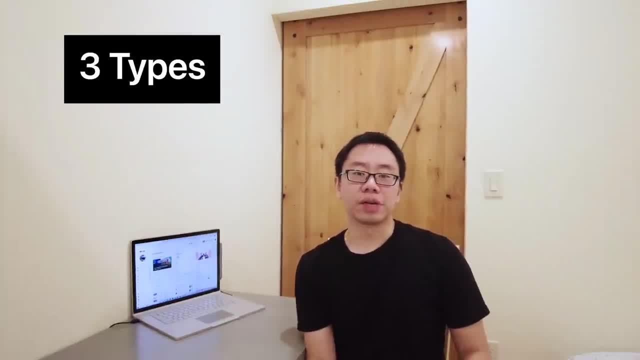 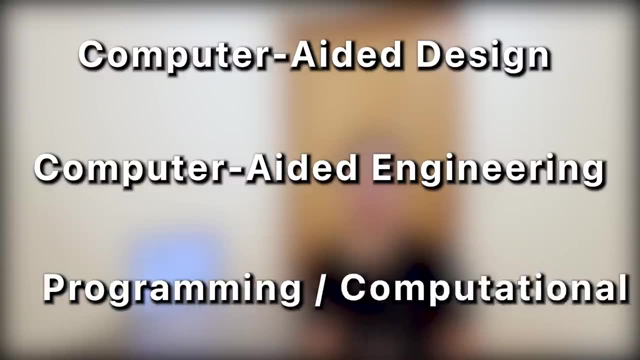 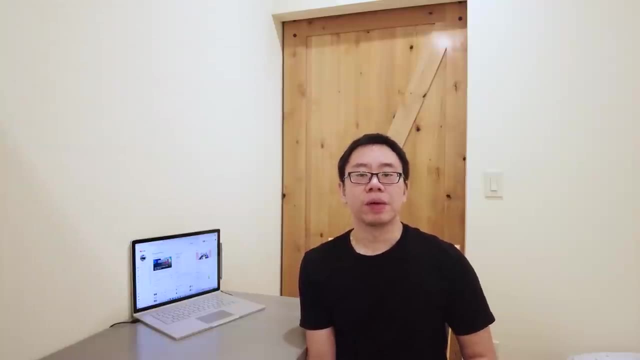 So in this video we covered three categories of software, including computer-aided design or CAD software, computer-aided engineering or CAE software, and computer engineering software For CAD software. learn either SOLIDWORKS or CREO or even both, And if you want to become, 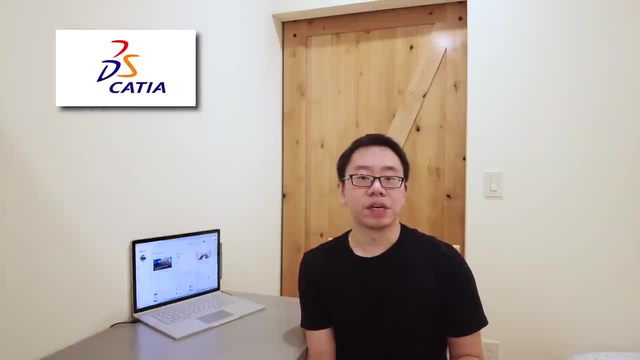 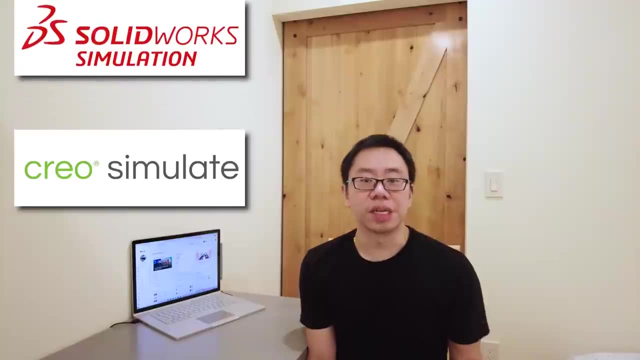 an automotive or aerospace engineer, definitely check out CATIA or NX For CAE software. start out by learning SOLIDWORKS or CREO simulation And then, if you want to take it a step further, learn ANSYS or ABTIS, If you know how to model problems involving 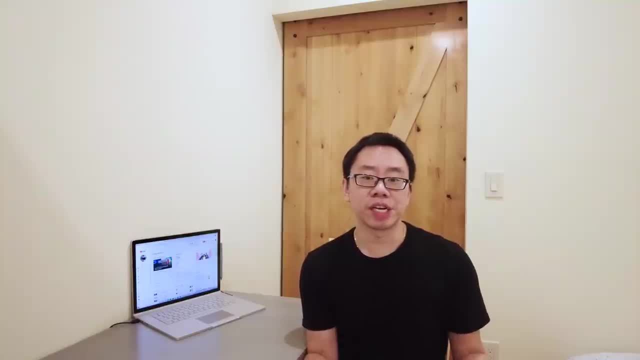 both solids and fluids. that's going to be a huge game-changer in your job search. Let me tell you, not many of you are going to be able to do that, But if you know how to do that, you're going to be able to do the job. 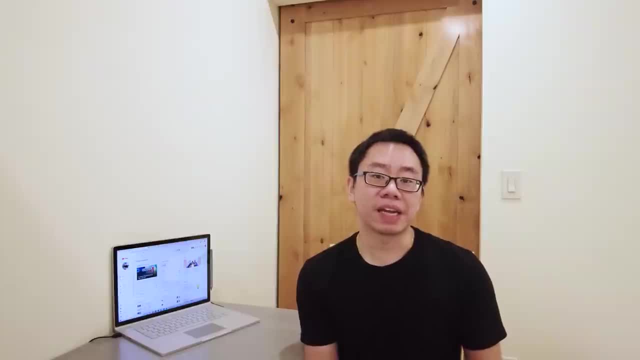 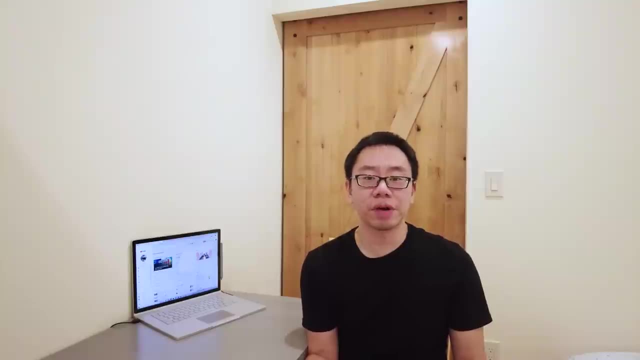 For programming. it's not a must-have skill for mechanical engineers like CAD or CAE software, But it's going to make you very competitive and efficient. So if you have the opportunity, definitely learn Python or MATLAB. And then for statistical analysis software, both JUMP and MINITAB are very capable and 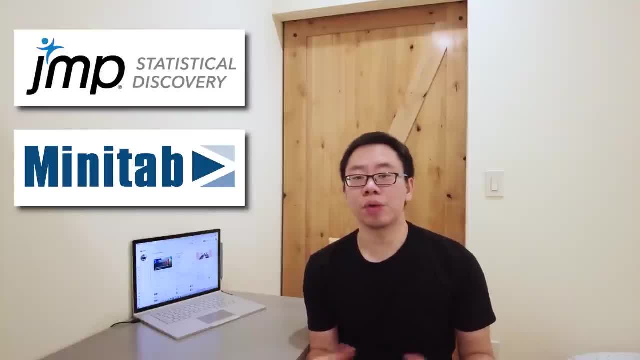 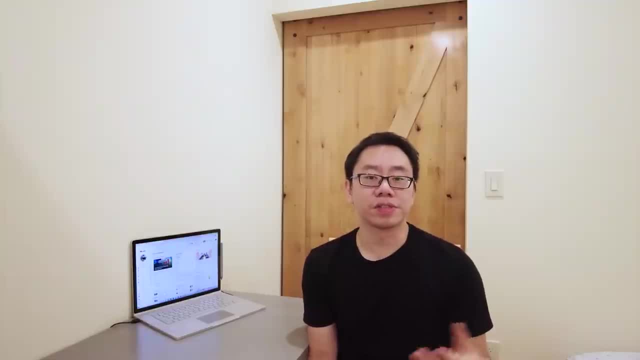 it's likely you have to use them at some point in your career, so it won't hurt to pick and more. Finally, we talked about graphical programming software, and if you want to design control systems, learn Simulink. And if you want to test products and automate processes, learn 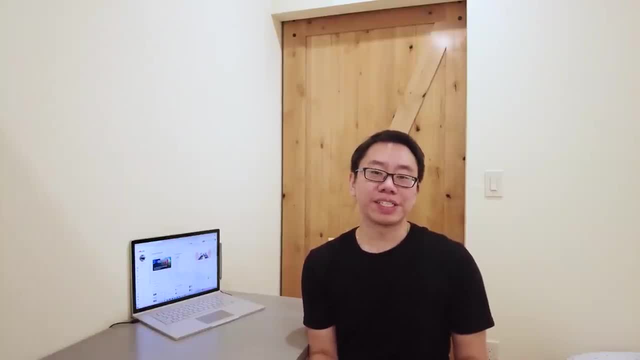 LabVIEW. Alright, that's it for today's video. guys, As always, thank you so much for watching And if you enjoyed this video, please like and subscribe, And let me know in the comments below if I missed any software that you think mechanical engineers need to know, And I'll. 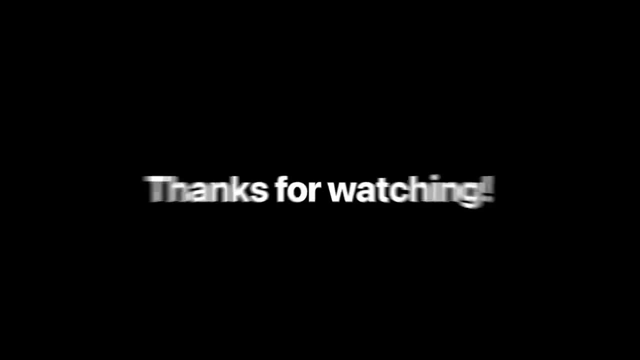 see you in the next one. Peace, Bye, Bye.